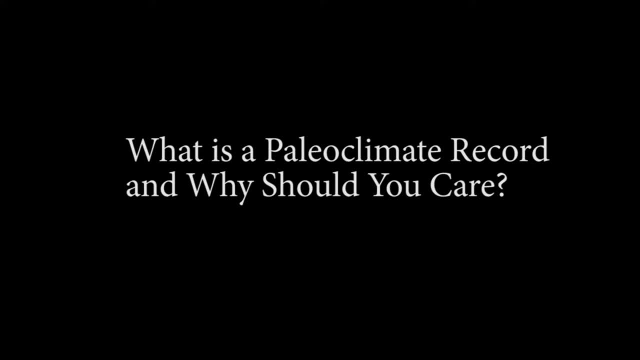 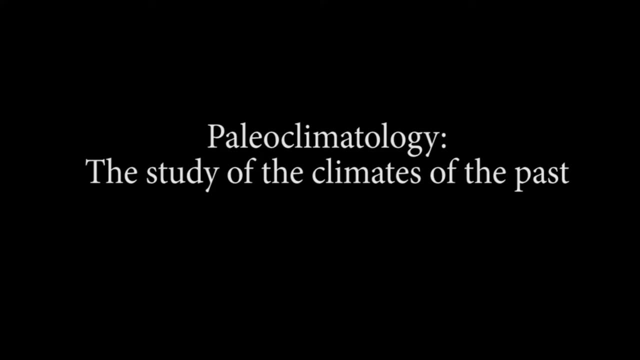 So what is a paleoclimate record and why should you care? First I'll say a little bit about what paleoclimatology is. Paleoclimatology is the study of the climates of the past. Paleoclimate records consist of a lot of efforts. 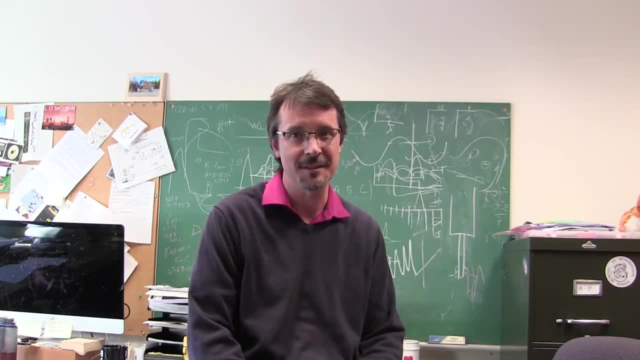 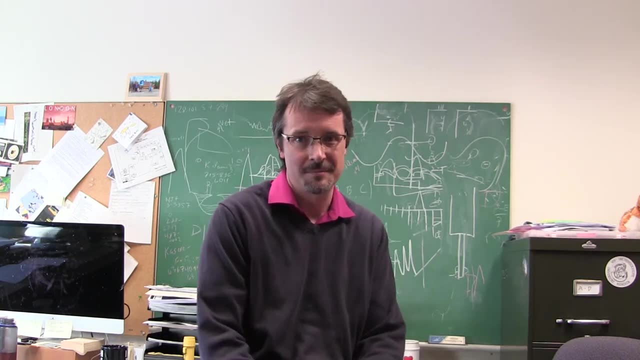 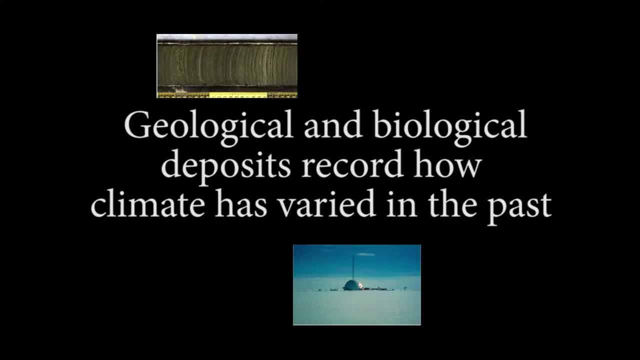 by geologists and ecologists and other scientists to go out and identify different kinds of deposits on the Earth's surface, be it ice cores, marine sediments, corals, tree rings, lake sediments, all kinds of different geological deposits or biological deposits. 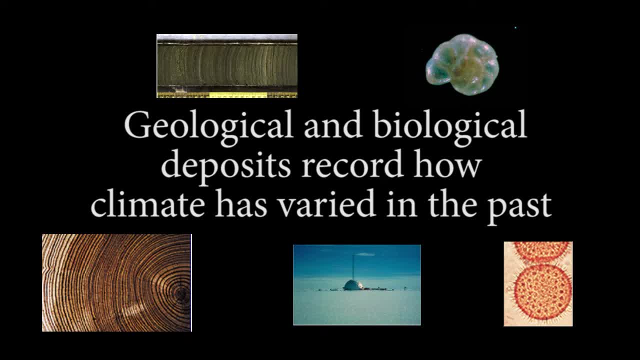 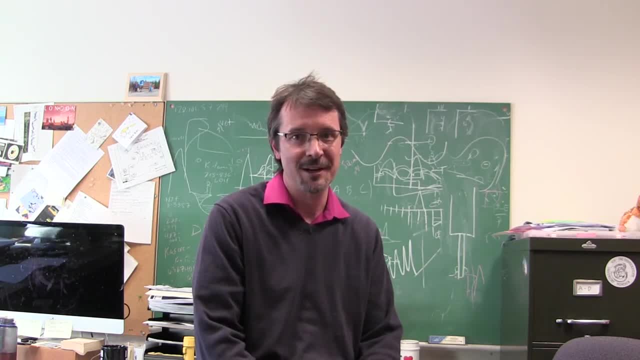 that record how climate has varied in the past. It's a really, really diverse science, which is why I enjoy it. In my work I get to go into tropical Africa, Indonesia, other places take long sediment cores or other types of geological archives. 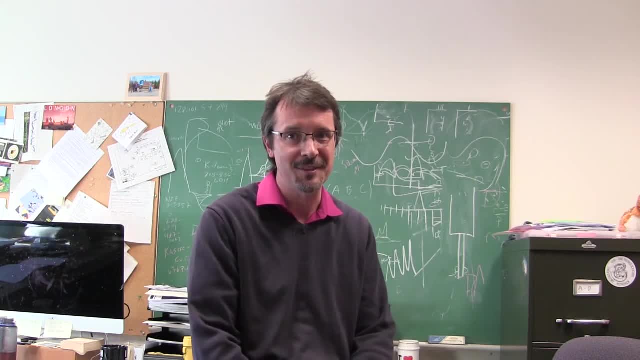 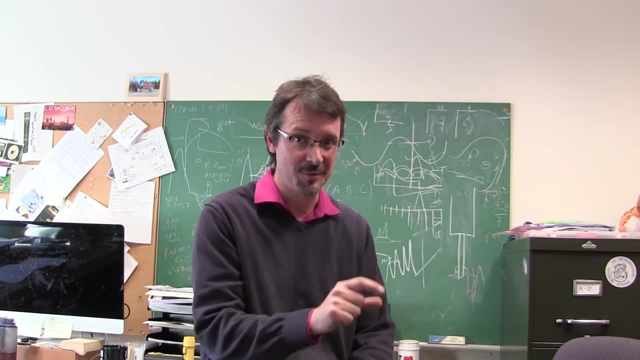 and bring them back to the lab and measure all kinds of different things in them, Everything from the pollen that they contain, that tells us about how vegetation changed in the past, to measuring the chemistry of those sediments, which can tell us a lot about changes in temperature and the hydrological cycle. 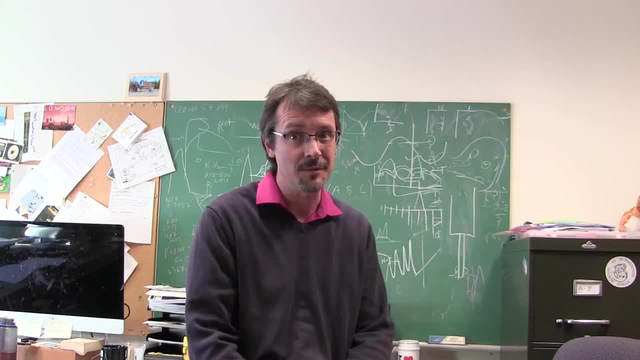 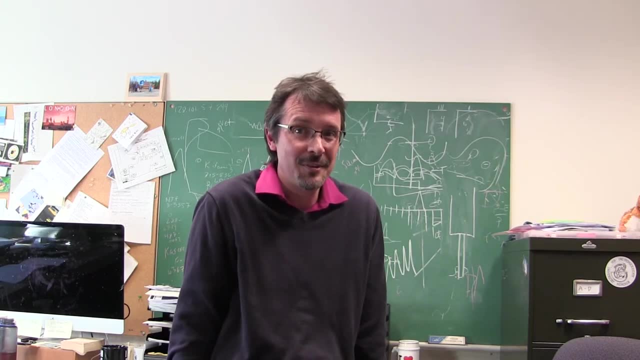 So paleoclimate records consist of lots and lots and lots of different deposits, like those that tell us about how Earth's climate has varied through time. Why should you care about that? Well, there are many reasons to care about Earth's history, Whenever you hear. 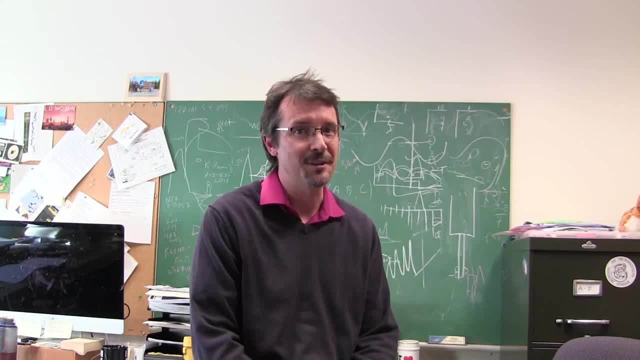 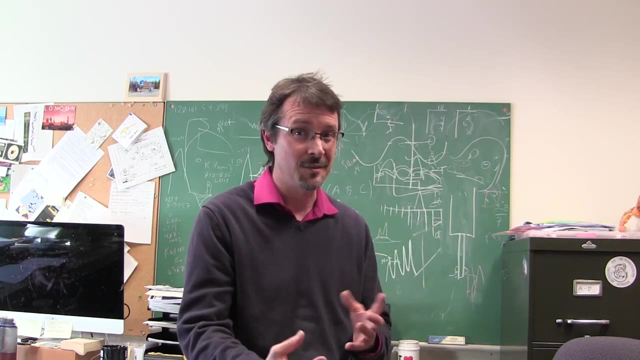 someone say the Earth is now warmer than it has been in a thousand years, they're referencing efforts by hundreds and hundreds of paleoclimatologists to go into these geological archives and reconstruct temperature and compare those temperatures against the modern. So in essence, the paleoclimate record lets us 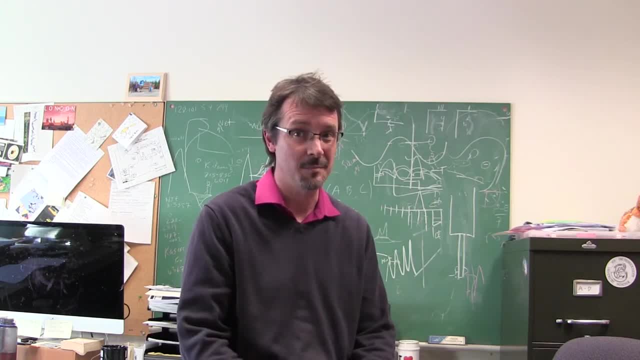 investigate climate on timescales much longer than anything that people can observe. We have weather station data that extends back maybe a hundred and fifty years in the best case. This is a very, very short time period to understand the full workings of our climate system. 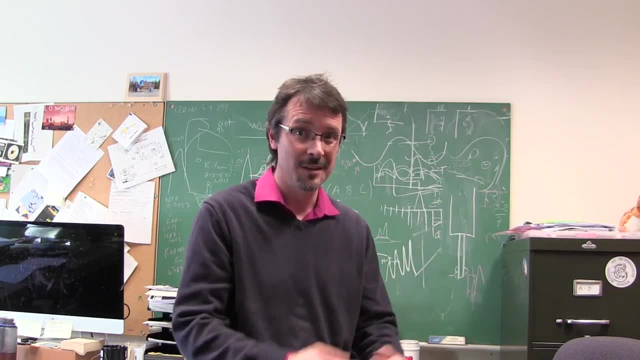 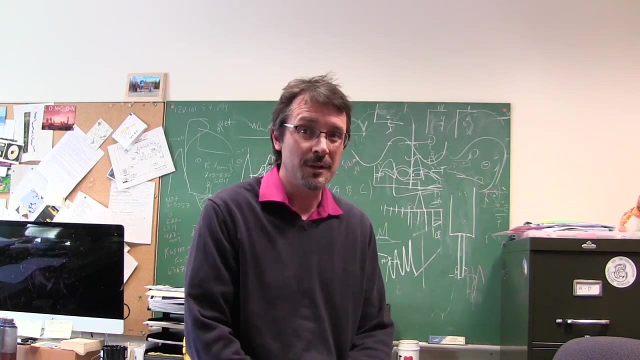 Paleoclimate lets us access those much longer timescales to try to understand and contextualize the climate changes that are occurring today. We can do several things with those records. Not only can we contextualize current climate change, the paleoclimate record provides one of the only